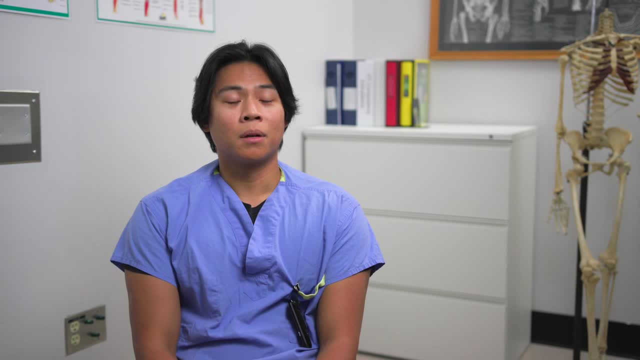 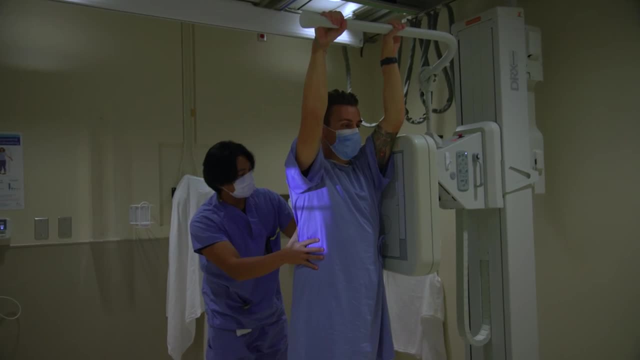 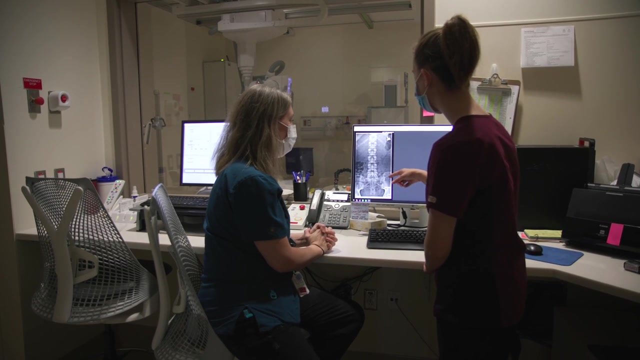 would be a good fit for those who are both social and are interested in caring for others, because a huge part of our job is patient care and patient interaction. Well, the program that I'm taking, which is the x-ray program, so that one is two years, so it's. 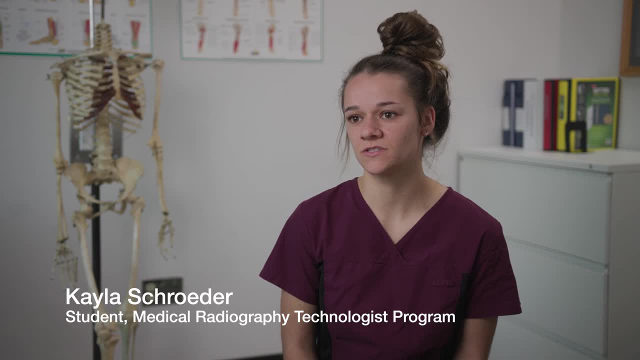 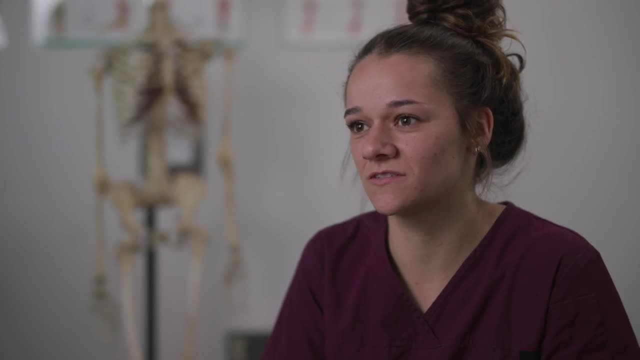 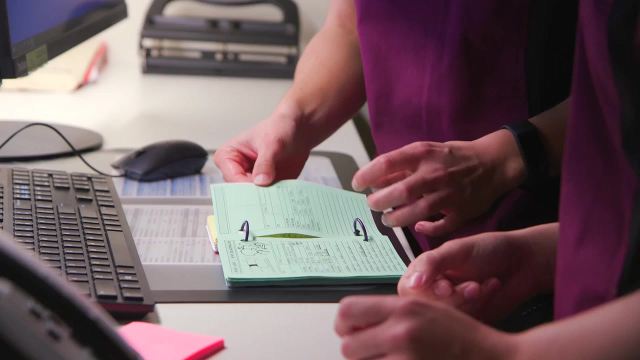 consecutive, so it just keeps going. so for two full years go throughout the summer. It's hard but you get used to it and then once you start your practicum, it really all starts to make sense. This program and it just kind of is just general x-ray, so I could branch off into CT mammography. There's quite a few. 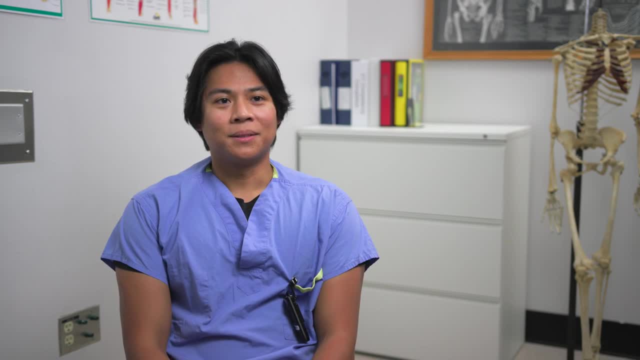 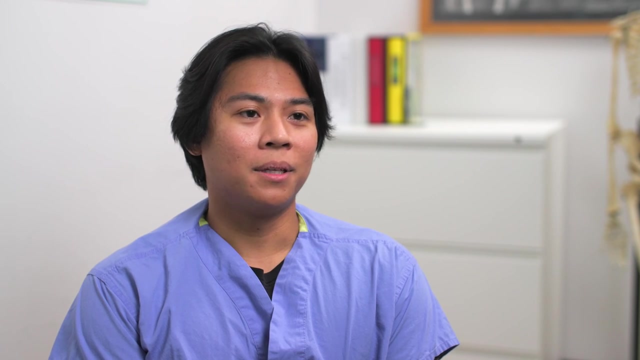 things I could branch off into. When you do your clinical practicum at a site, especially if it's your last level, it does almost serve as a an interview process, because this is when they start seeing your work ethic, how you fit into the department. it is indeed like a long interview process at that point. As a 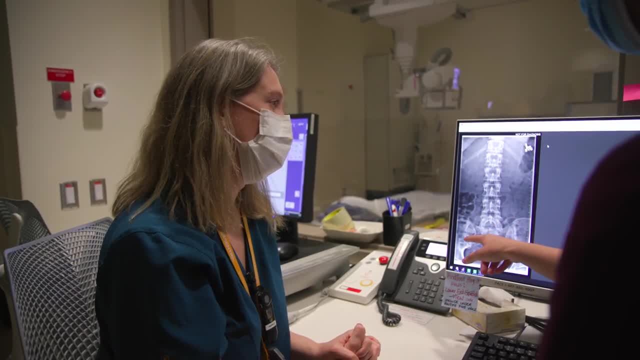 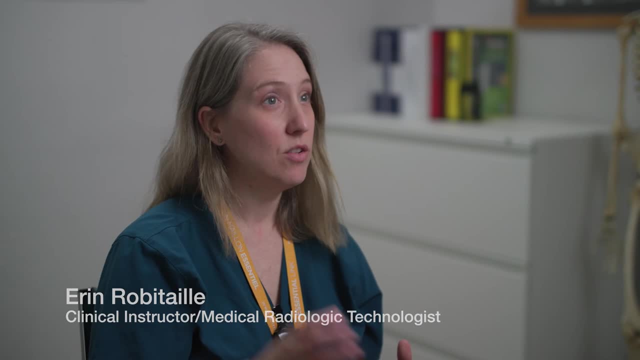 clinical instructor work with all the students going through the medical radiation program when they come out on their practicum. so my job on the floor with them is to ensure that they're learning the skills that they learned in school and turning it practical sense and that they're going to be tech ready when they graduate. You do have to have some 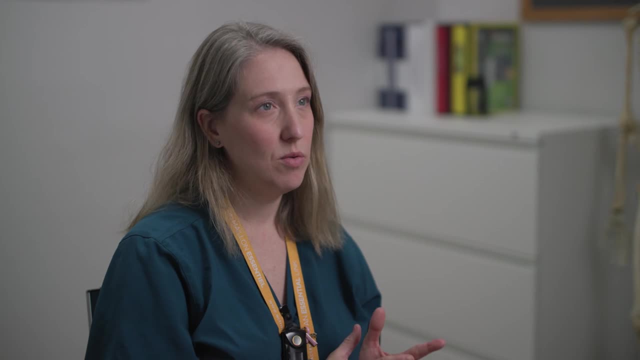 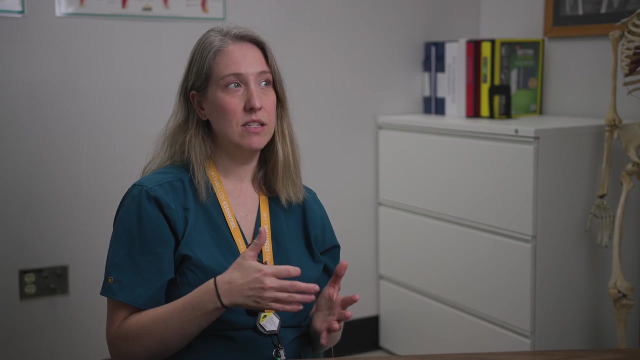 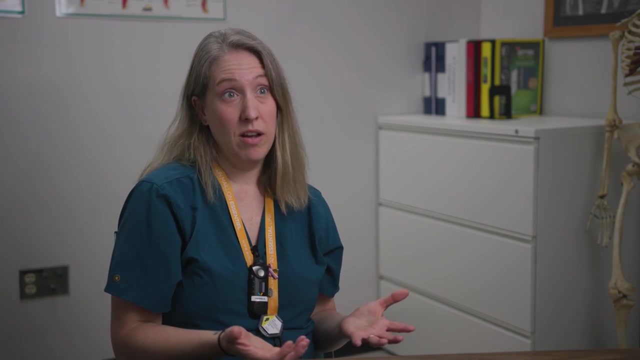 sort of sense of like book smarts. a lot of programs will want you to have like these high grades. but it's not always the book smarts that matter. it's your personality, it's how you can carry yourself when you're communicating with patients, because patient care is number one. that's why we're in healthcare. we're 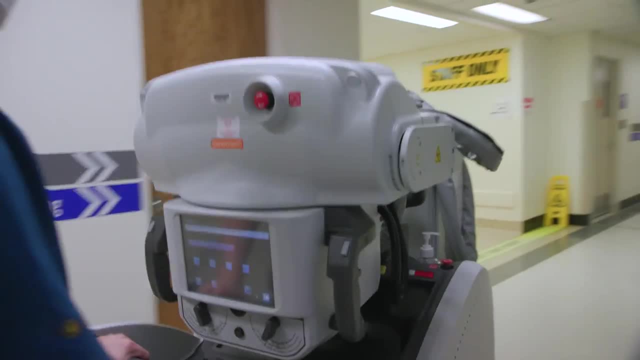 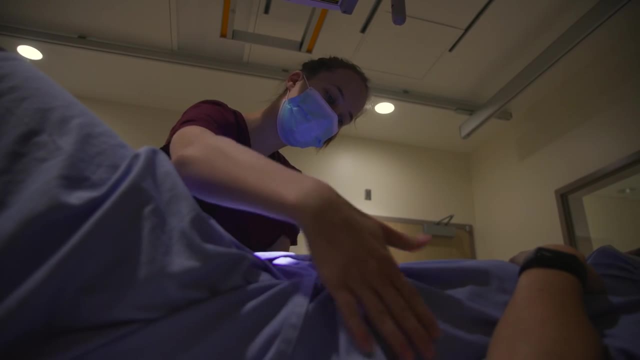 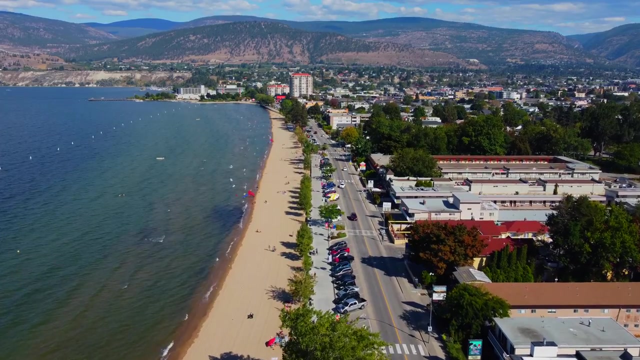 here to take care of people. Right now there is a high demand for that for the profession and we're only seeing an increase. our demand in the field is getting higher. The wage is actually really great. to be honest. Wage wise, there is definitely a lot of room to grow. The work-life balance can be amazing. two: lakes on either side. I live five minutes from a lake right now, so for me I get off work at four and I'm down at the beach by five. I love living in a small town, being nestled between two lakes, because in the summers you get your. 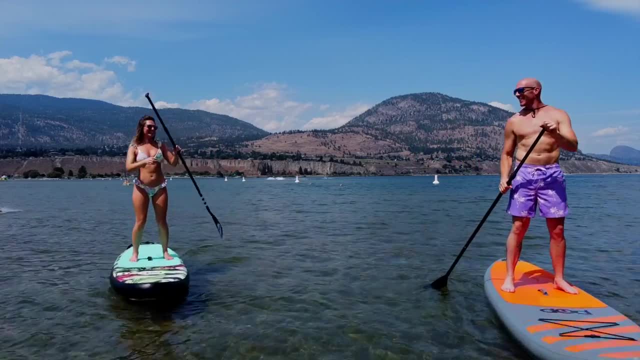 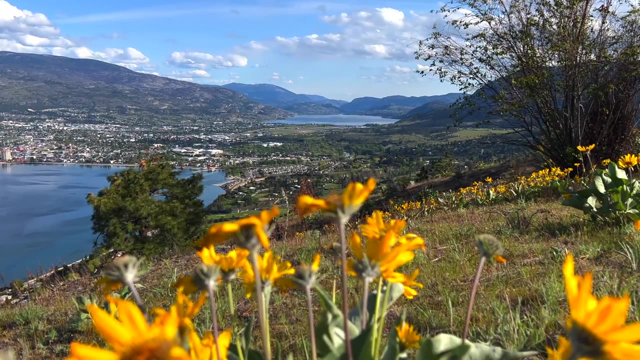 choice of lakes to go into, go swimming or paddle boarding, go kayaking. there are tons of hiking trails around. In a full-time position, you start with four weeks holidays. Vacation is one of the perks of the career. so when I first started I started off as a casual and then I got a part-time position. I